field of a black hole. the vacuum becomes unstable and these fluctuations start actually producing particles. So a fluctuation would normally be such. maybe an electron and positron could be spontaneously created, but then they would annihilate again because they cause some energy And by the uncertainty principle, if you have some energy it can only live for some time. 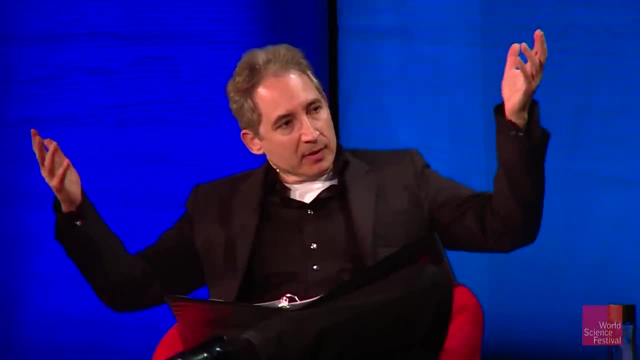 That's the fluctuation. So if those particles fly away, they appear as So now the gravitational field of the hole. they're still created by quantum fluctuations, But before they can re-inhalate. they're still created by quantum fluctuations, But before they. 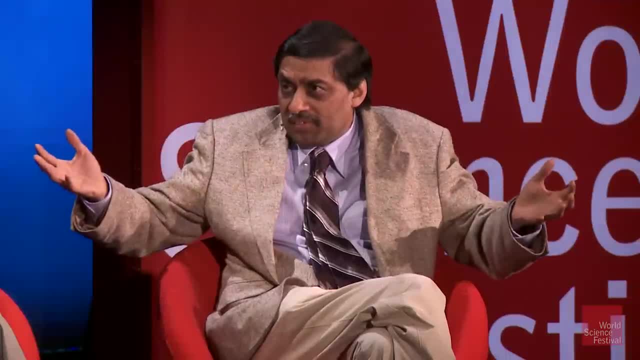 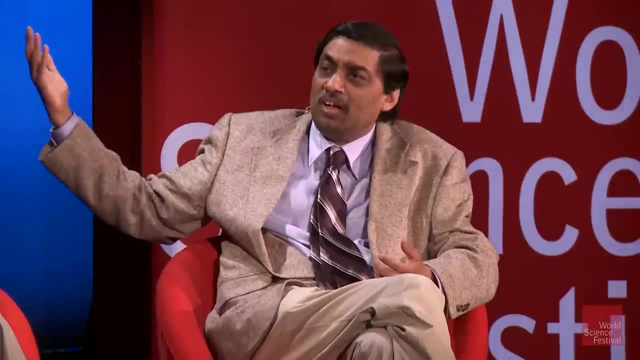 can re-inhalate. they're still created by quantum fluctuations. But before they can re-inhalate, the field of the black hole pulls them apart And one particle falls in the hole. but one manages to escape And the guy who escapes is called the radiation from the black hole. 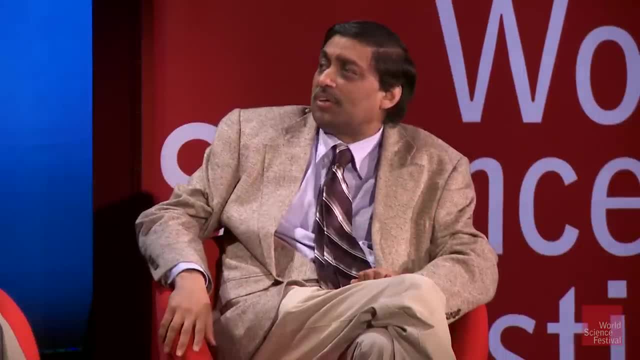 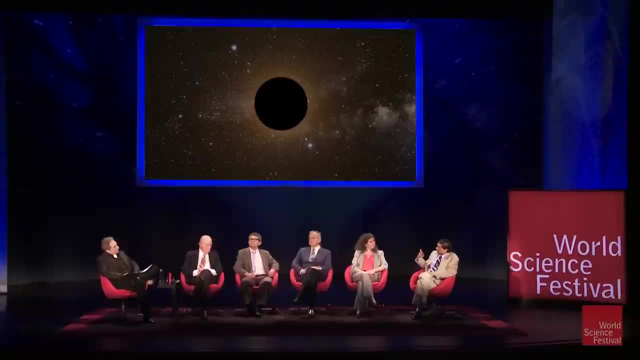 And this is what Stephen Hawking found, somewhat to his own surprise, in 1974, that black holes are actually very gently and very slowly, but because of quantum reasons they are always emitting something And as the black hole gets smaller, because it's sending stuff out. what happens to the strength of the radiation? So the radiation actually becomes stronger and stronger. It's just a matter of scales. A black hole has just one scale in it: the size of the black hole. So if you ask what's the wavelength of the radiation it emits? 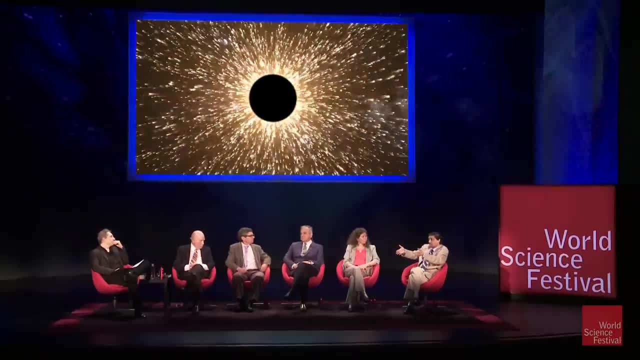 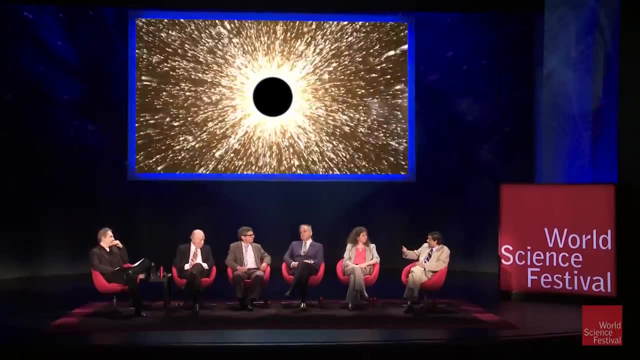 it's the same as the size of the black hole. And now that's really interesting. as the hole gets smaller and smaller, the wavelength emitted is also getting smaller and smaller, which, as you know, means it has high and higher energy. So it's going to end. 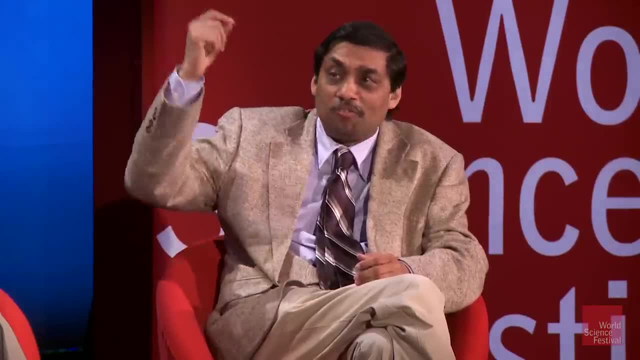 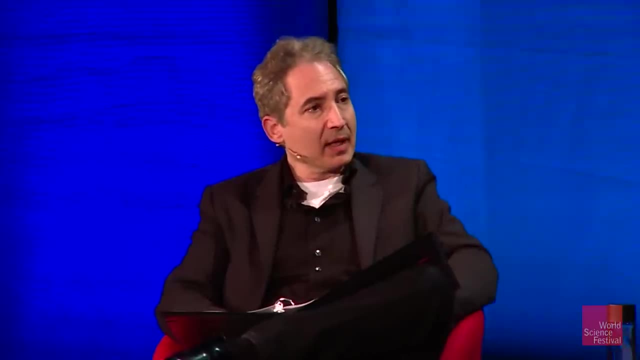 up in an explosive thing at the end. It's going to sort of just squeak off to an end. Well, you can see it happening there. So, in short, black holes have a positive energy. holes are not fully black when you take quantum mechanics into account. Now, this I mean. 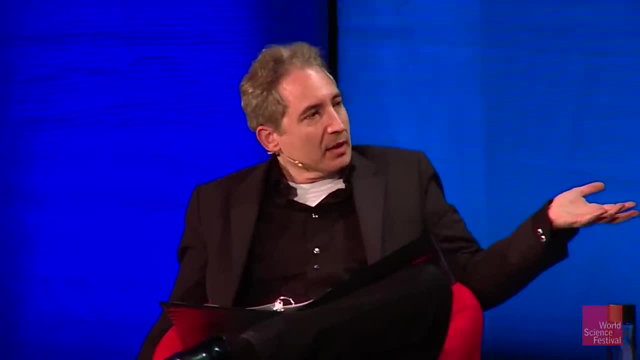 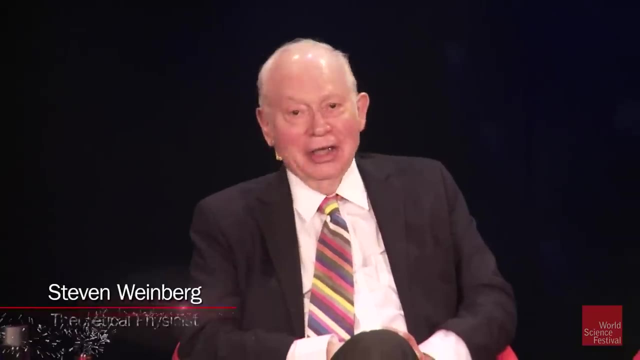 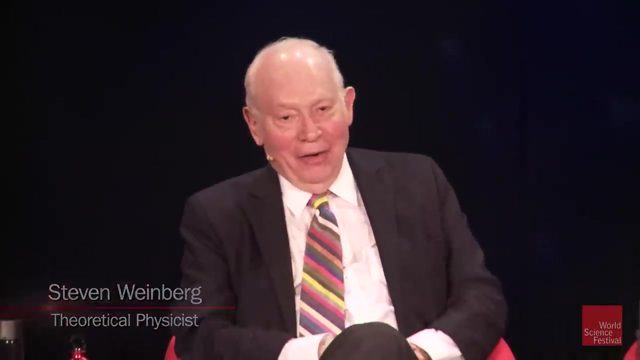 I wasn't around at the time. It must have been a huge shock. Steve, was this a shock to you? Yes, At that point I was still hoping black holes didn't exist, which would have had the tremendous merit that I wouldn't have had to understand the Hawking theory. But I'm 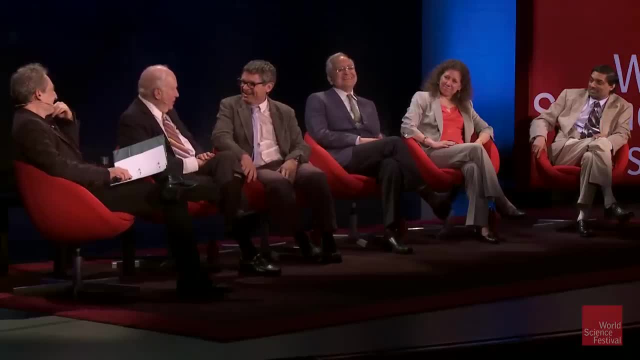 afraid I've had to live with it. 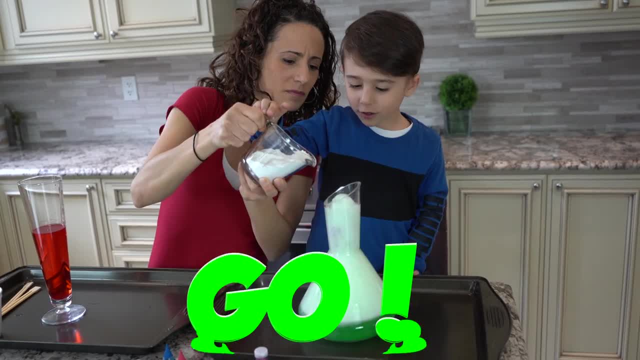 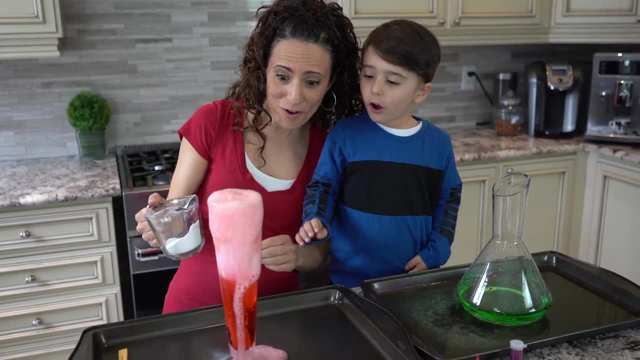 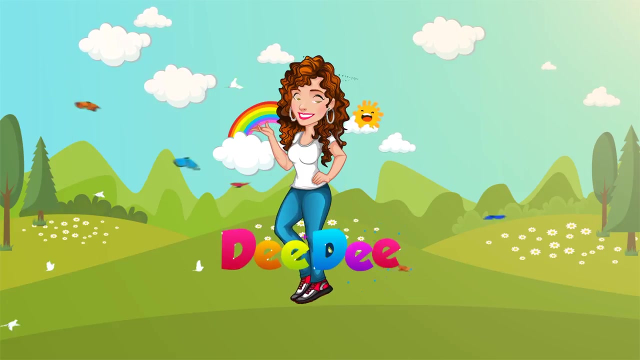 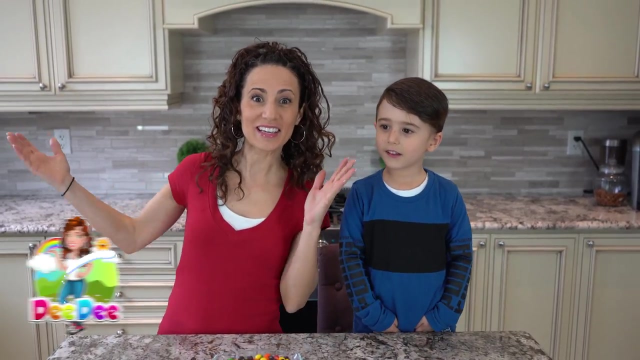 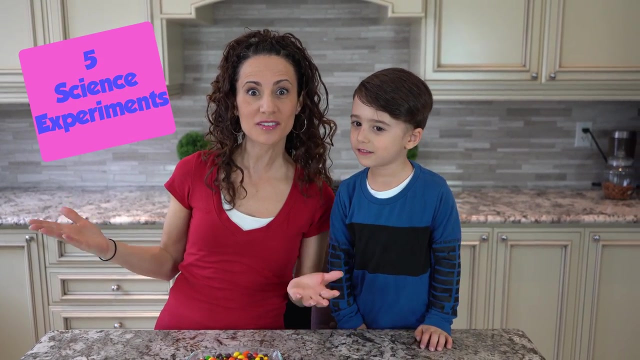 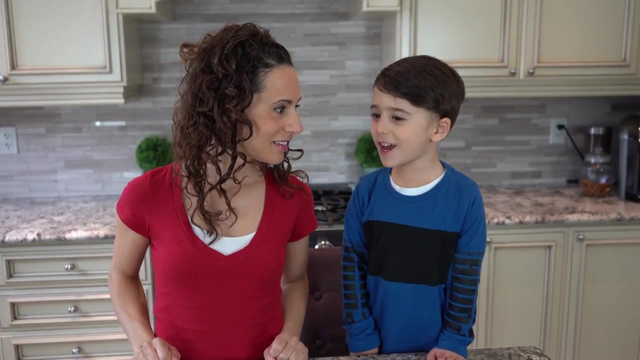 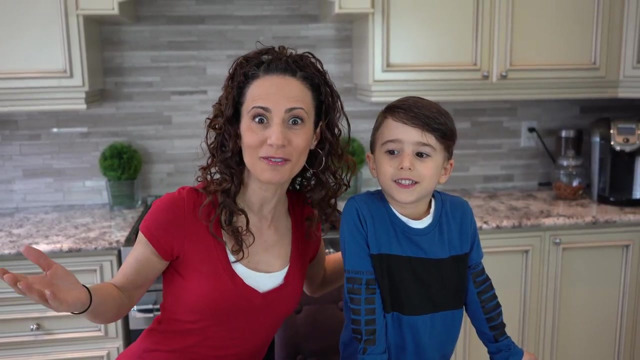 One, two, three go, Explode, Volcano, Volcano. Let's get together, run and play with DeeDee- DeeDee. Hey, kids, it's me, DeeDee and Mateo. Yeah, today we're going to do five different science experiments at home, with all the stuff you have inside your house. This is going to be a lot of fun. Are you ready? Yeah, But make sure when you do these experiments, kids, you have a grown-up to help you. So I'm here to help Mateo do them. Let's start these experiments, Yeah.